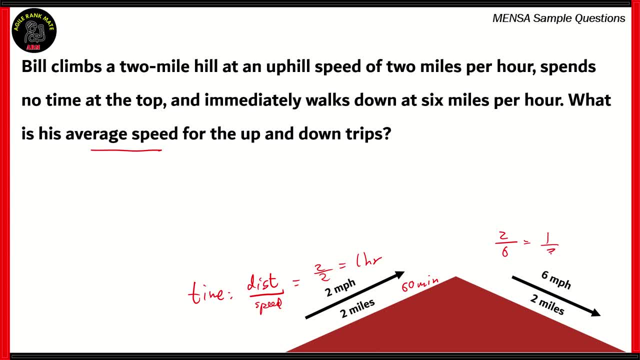 completes the descent in a third of an hour. Now, since one hour is 60 minutes, a third of an hour would mean that he completed the descent in 20 minutes. So therefore, the total time that he took to climb up and down the hill is 80 minutes, And we know that the total 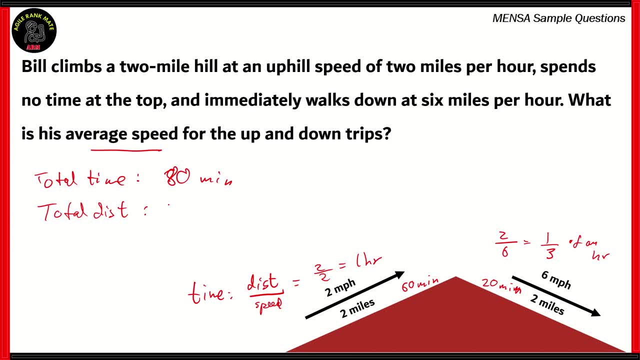 distance, which is 2 miles up and 2 miles down, would amount to a total of 4 miles. So, in order to find out the average speed, that's what we need to divide. We need to divide the total distance traveled over the total time taken. 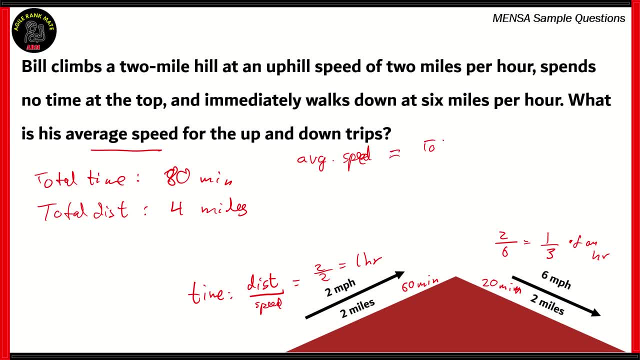 Okay, So average speed is total distance upon total time, which is 4 miles over 80 minutes. Now 4 miles are done in 80 minutes, so 1 mile would be done in 20 minutes because 4 goes into 80 20 times. 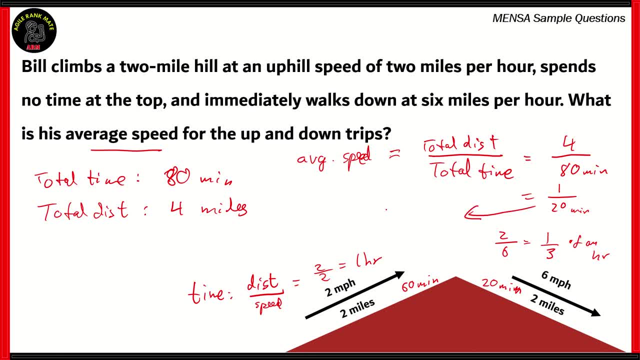 So 1 mile is completed in 20 minutes. So therefore, if you multiply both numerator and denominator by 3,, you get 3 miles completed in 1 hour. So therefore, the correct average speed is 3 miles per hour. The answer is 3 miles per hour. 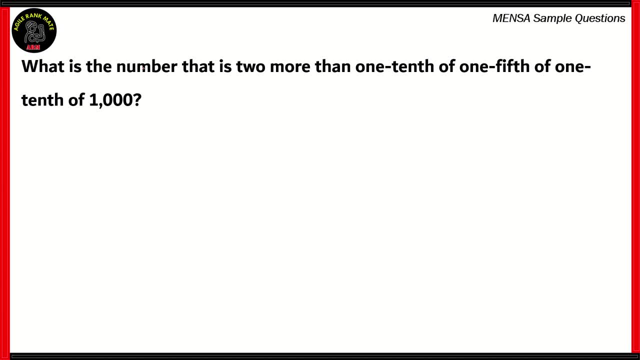 Now let's look at another question. What is the number that is 2? 2 more than 1 tenth of 1 fifth of 1 tenth of 1000.. Now, at first glance this looks like a very complicated question. However, we can solve it real easily. Now, 2 more than. 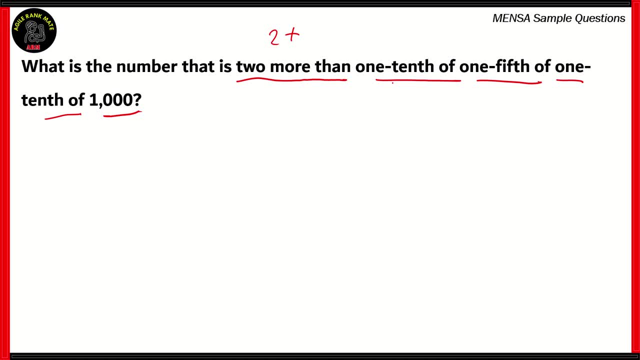 means that 2 is added to a number And that number has something to do with 1000.. So 1000 is the numerator. Now we have to multiply 1 by 10,, 1 by 5, and 1 by 10. And then that product is multiplied. 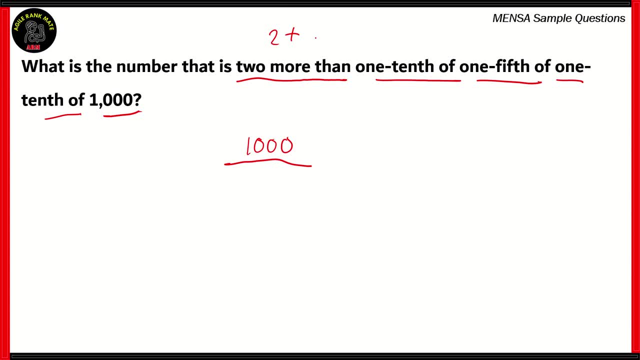 with 1000 to get a certain number that is added with 2.. Now the idea is, in order to solve this question, we need to start backwards. Now what does that mean? That means we need to start from 1000.. 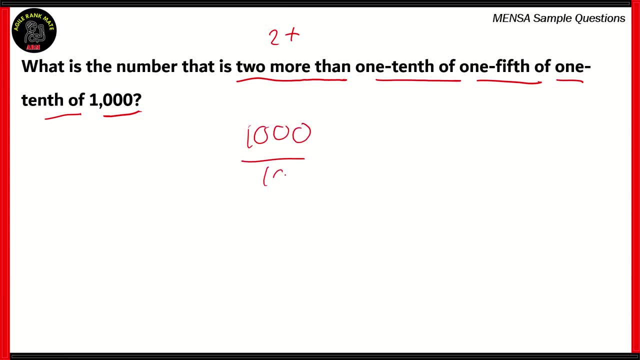 So we need to find a tenth of 1000,, which is 100.. We need to find a fifth of 100, which is 20.. And then we need to find a tenth of 20, which is 2.. So you can do it this way. 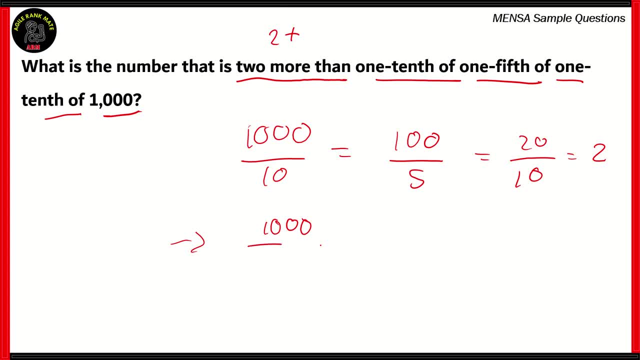 or you can just put in all the denominators together at once, because the word of in Bod Maths actually means multiplication. So you can multiply all these fractions of 1000 that you need to get. So 1 by 10 times 1 by 5 times 1 by 10 gives you, you know, it gives you 500.. So 1000. 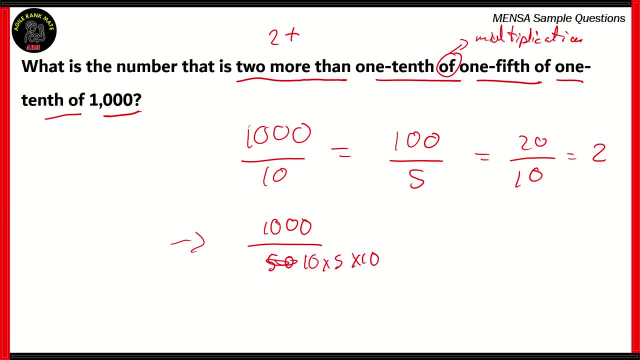 over 10 times 5 times 10.. You can cut out the zeros, So you get 10 over 5, which is 2.. Now the original number we're looking for is 2+, The division of 1000 by 500. So therefore, that is 2.. So therefore, the answer is 2. 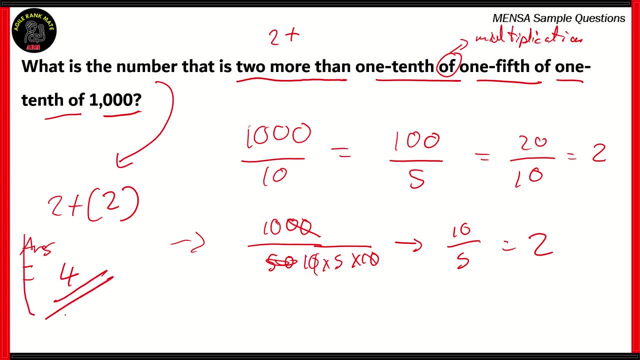 plus 2, which is equal to 4.. So, therefore, the right answer for this question is 4.. Now, in case of multiple operations, we will follow the Bod Maths rule. Now, over here we have division and addition to be done, So we did the division first. 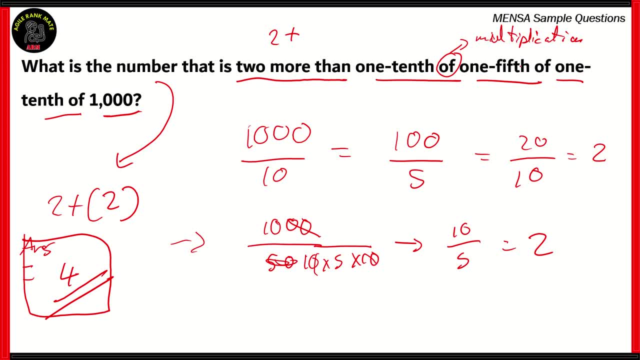 Now, in division, all of these percent, all of these you know fractions, are to be taken out of 1,000. So we combine them together to form 1 by 500 of 1,000, which is 2.. And that 2, when added with another 2, gives you 4.. So 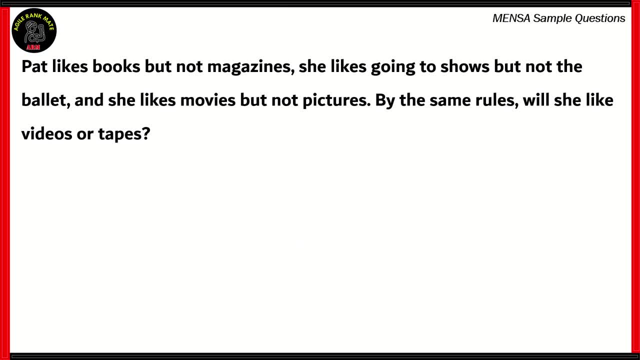 therefore, the right answer is 4.. Now let's look at a verbal problem. Pat likes books but not magazines, She likes going to shows but not the ballet, And she likes movies but not pictures. Now, by the same rules, we need to find out whether she likes videos or tapes. 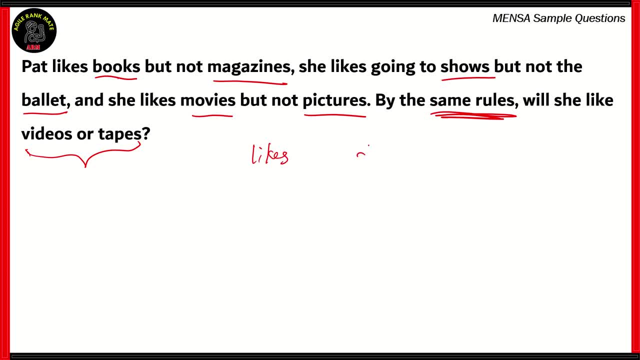 Now, in order to do that, it's a good idea to classify her likes and dislikes. So her likes include books, shows, movies, And her dislikes include magazines, ballet pictures. Now, if you look at the likes, you can see that Pat likes books, she likes shows. 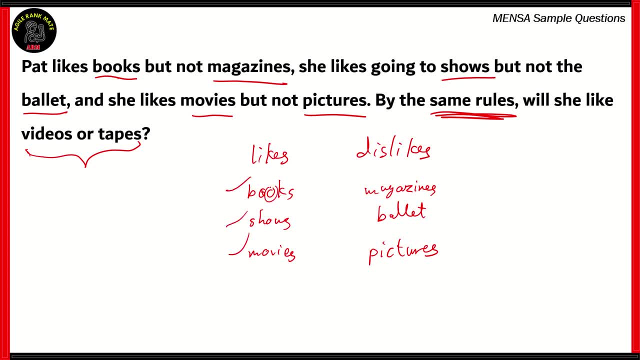 she likes movies. Now, as you can see, all of them contain at least one O in the word. There are two O's in books, one O in shows as well as movies. So, therefore, um, the rule that Pat uses to like something is whether the word has an O in it, At least one. 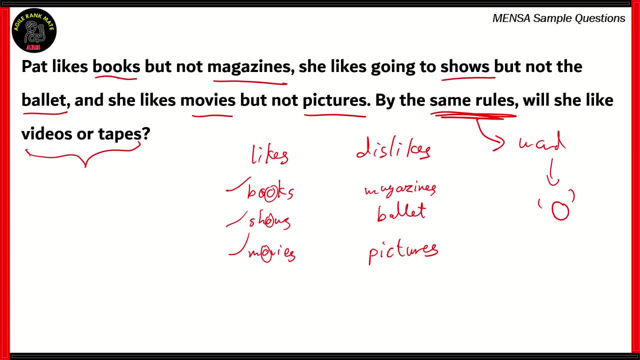 O must be present in that word. So therefore she will like the hobby or the product. So when it comes to videos and tapes, we can see that videos have the letter O in it. The word videos has the O in it, So therefore, uh. 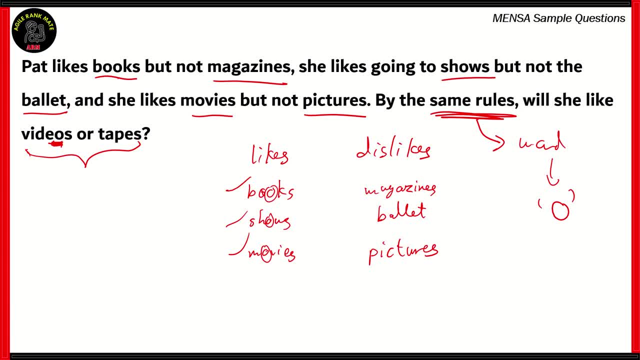 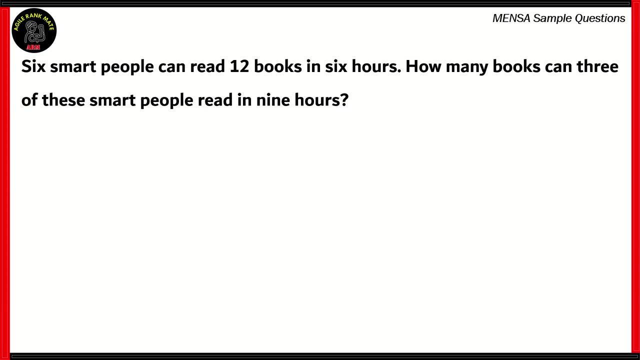 according to the same rules, Pat is supposed to like videos, So the answer here is videos. Now let's look at an important question. Six smart people can read 12 books in six hours. How many books can three of these smart people read in nine hours? 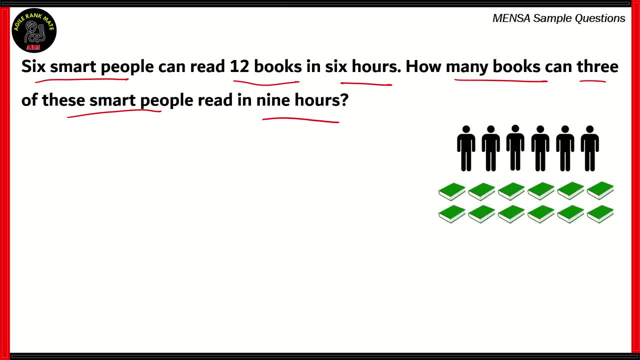 So, in order to visualize what we're dealing with, here is an illustration. So we have six people, we have 12 books and the 12 books are completed by these six people in six hours. So we need to find out how many books can three of these people read. 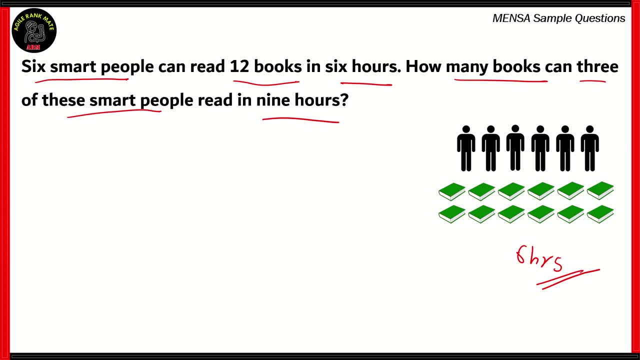 in nine hours. So we need to find the number of books read, if the number of people and time are given. So that means we need to construct a number of books, So we need to construct a number of books. The following: six people in six hours complete 12 books. Now we would need to find out how how much a person reads in. 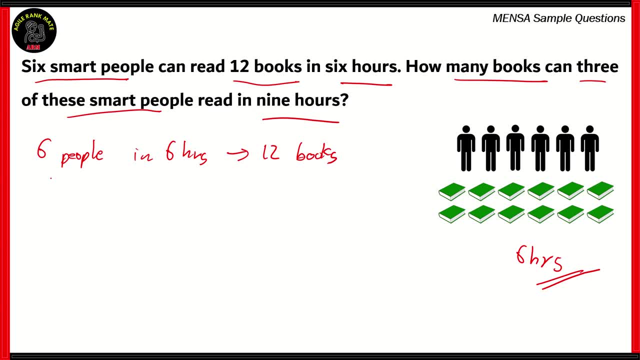 an hour. So when we divide the number of people so you get one person in six hours reads twelve by six, which is one person starting at eight days seems less than one person starting at 12.. And if we include that number and divide it by seven, we'll see that 12 takes one account into the second account. So, in other words, a five person equals 12 books, So some people can read 12 books twice an hour, familiar to me here in the video. Now let's really use some basic magic tricks to try So we can divide these numbers in order to specify the number of books we get programs. 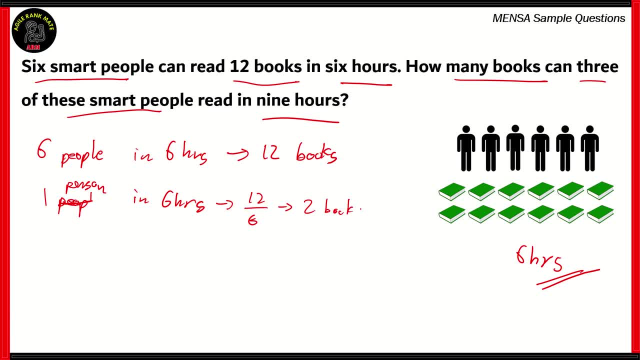 We don't have to go here to number six books. Some seem to be just several four book inflammatory books. other people can just do a magic challenge and put them and some littleık is two books. So if you are looking at one person, one person would deal with two books. 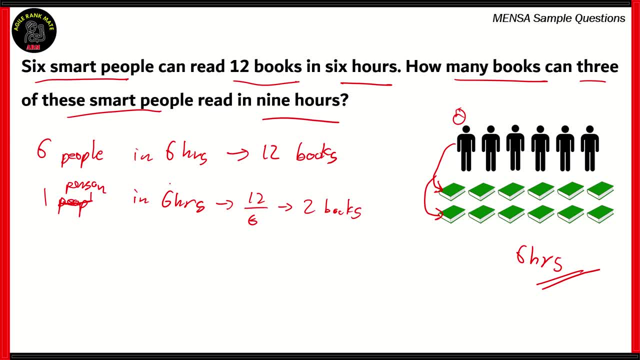 during the six hours time period. Now if we were to find out how much that person reads in an hour, so one person in one hour would read 2 over 6, which is 1 by 3 books. So one person would read a third of a book in one hour. Now this is the rate of the work done. 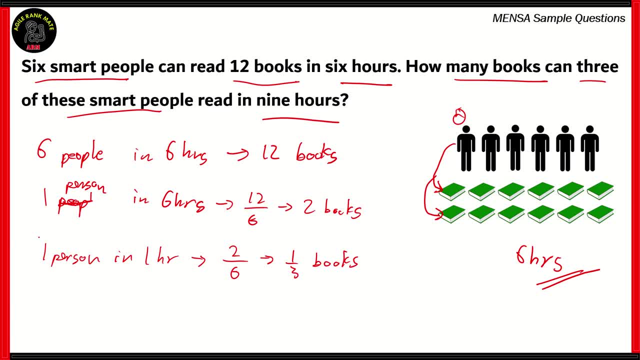 here Now we can use that rate in order to find out how many books can be read by three people in nine hours Now. three people in nine hours Now. we know that the rate of book reading is 1 by 3 books by one person per hour, So we're going to multiply that rate with the number of people. 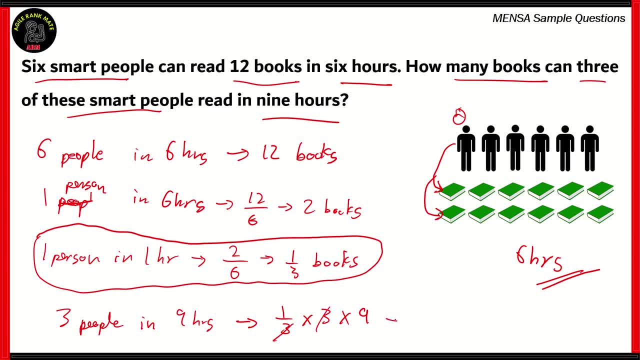 and the number of hours. So 3 cancels out with 3.. What we have is 9.. So the right answer is: 9 books are read by three smart people in nine hours, So therefore, that's the answer that we get. 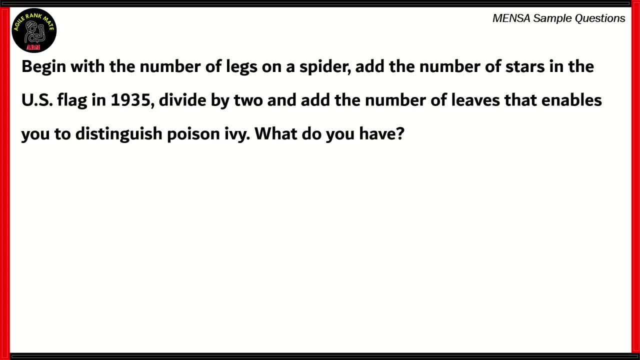 Now let's look at the final question for the day Now. here we have some objects from which numbers are taken and we need to find out a particular value. Begin with the number of legs on a spider. Add the number of stars in the US flag in 1935.. Divide by 2 and add the number of leaves. 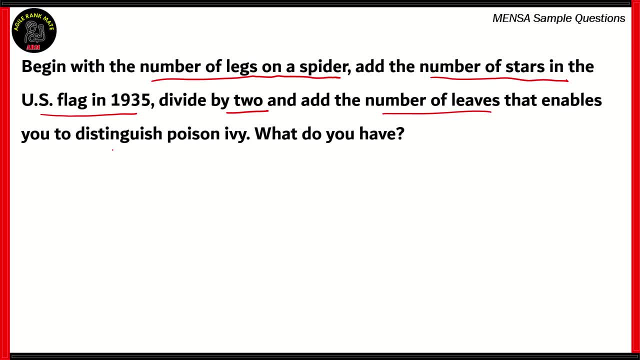 that enables you to distinguish poison ivy. We need to find out what is the resultant number that we get. So the number of legs on a spider is 8.. That's pretty obvious. But what about the other two? Now for poison ivy. 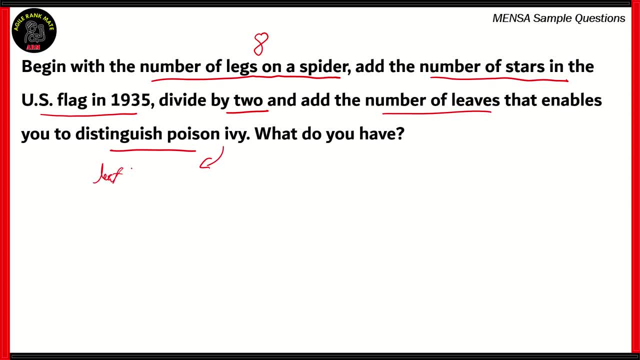 there is a popular saying that goes: leaflet three let it be, Which means that if you find a plant with three leaflets on a stalk, then it's best to avoid it, because it's most likely poison ivy. So poison ivy has three leaflets on a stalk. So that's how. so that's the number that we're. looking for. So eight legs, three leaves. Now, what's about the stars in the US flag of 1935?? Now, in 1935, we had the 48 star flag that flew from 1917 to 1959. So this flag was present till. 1959, when they changed it to 59 stars and then Hawaii joined the union and then they eventually made it two. I mean it was changed to 49 stars and then in 1960, Hawaii joined and then therefore, they had to make it to 60 stars. So the number of stars in the US represents the number of states that it. 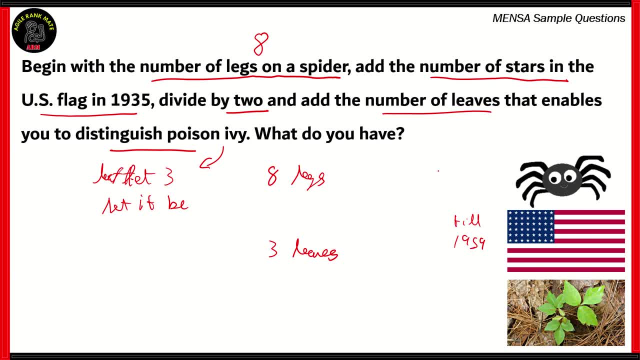 has. So in 1935, they had the 48 star flag. So therefore the number of stars is 48.. Now we need to first add the number of legs on a spider and the number of stars in the US flag. So that is. 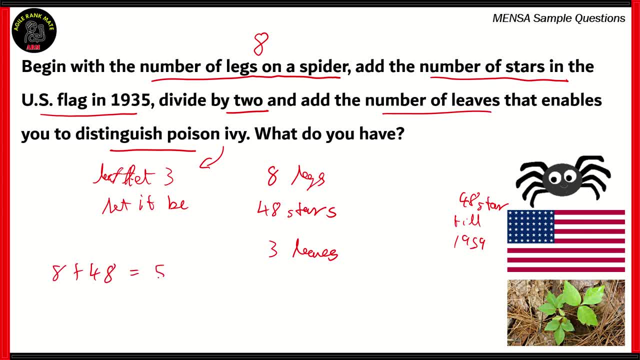 eight plus 48, which gives you 56. Next we need to divide that sum by two. So 56 over two gives you 28.. You can do that division over here. Two goes into five two times, but actually you get four. so 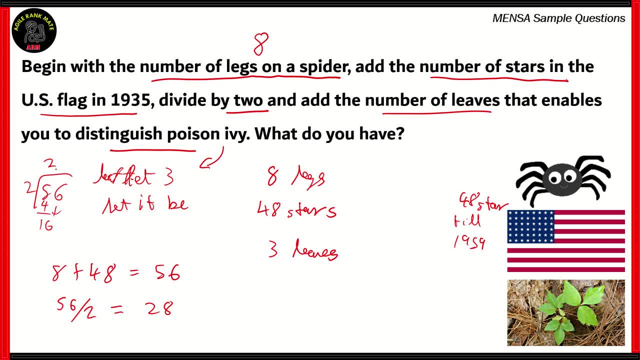 therefore one's the remainder, So six comes down at 16.. And two goes into 16 eight times. So therefore the quotient is 28.. So we have a quotient which is 28,. we need to add the quotient with the number of leaves used to distinguish poison ivy, which 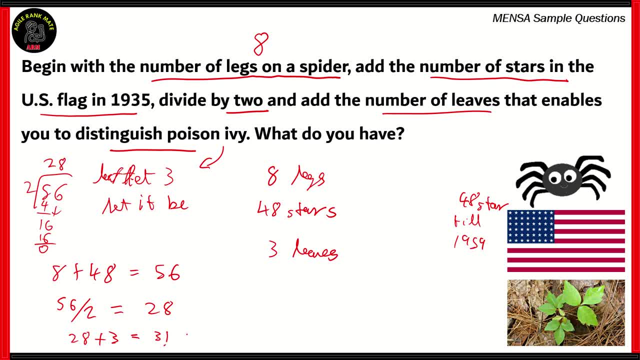 is three. So therefore, 28 plus three is 31.. So our final answer is the number 31.. So when you add the number of legs on a spider to the number of stars on the US flag in 1935, you get 56..